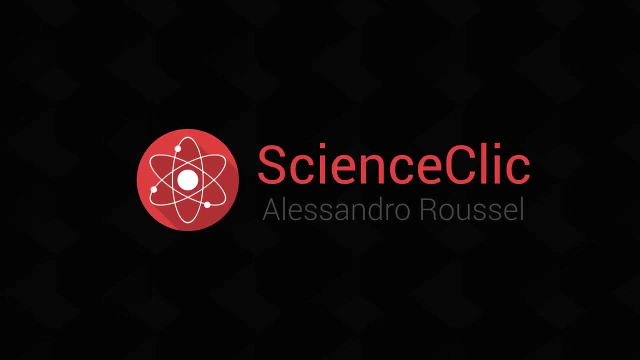 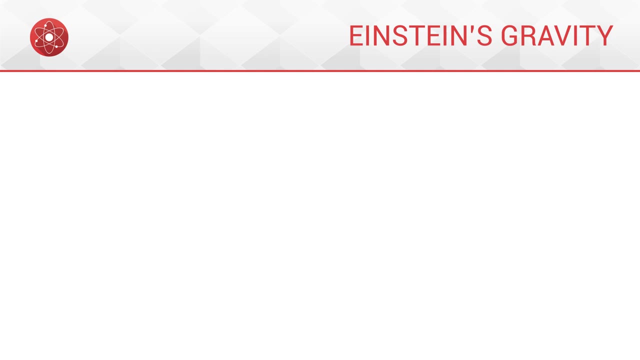 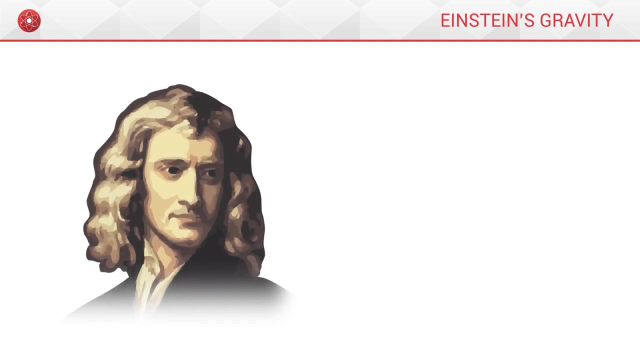 Welcome back to Science. Click Today Einstein's gravity. In the 17th century, Newton discovers universal gravitation. With this he manages to predict the movement of an apple falling from a tree or the orbit of the moon around the Earth. 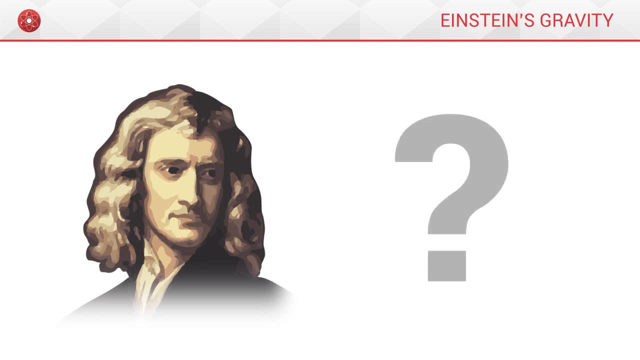 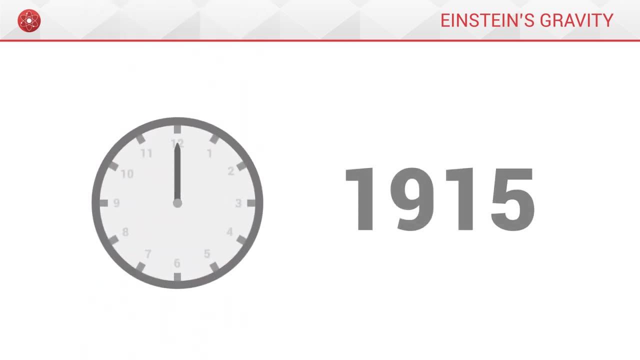 However, Newton does not manage to explain why gravity exists, nor how it acts. To answer these questions, it is necessary to wait for the early 20th century, with Albert Einstein's theory of general relativity. For Einstein, the three dimensions of space in which we move and time in which we evolve, 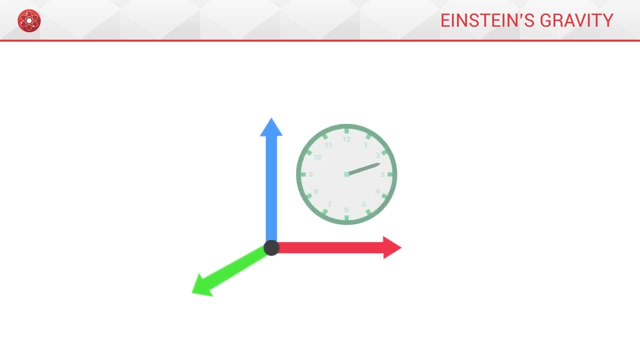 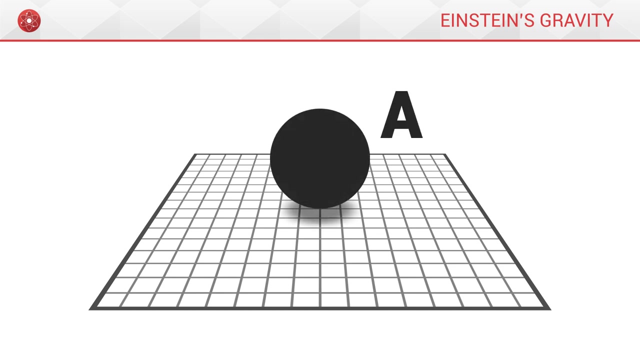 are just two parts of the same thing: spacetime. In spacetime, objects exist in a given place at a given time. Now let us try to conceptualise spacetime as a grid on which we could place an object: A. When A is placed on this grid, it distorts. 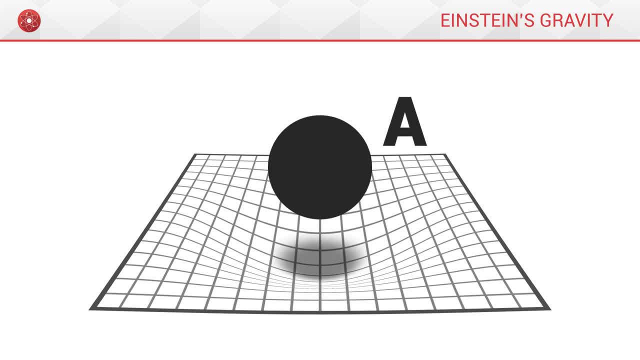 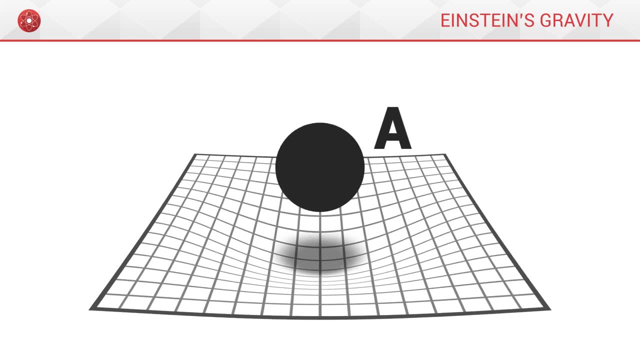 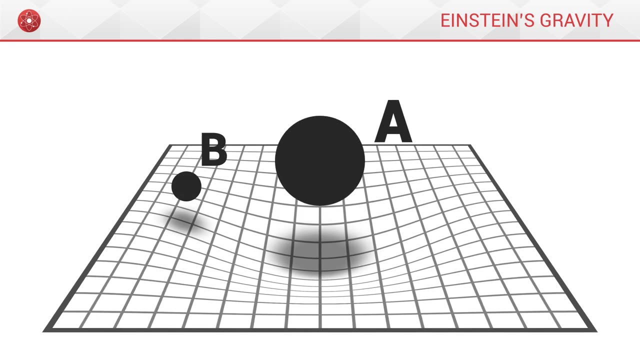 it according to its mass. The more massive the object, the more it will distort spacetime. Inversely, the less massive, the less spacetime will be disturbed. Now let us imagine that we place a second object B on this grid. B distorts spacetime as well. 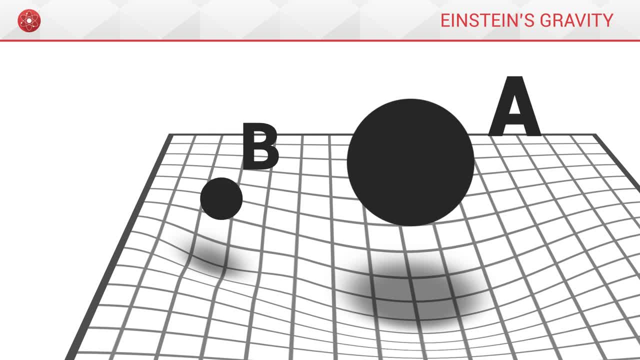 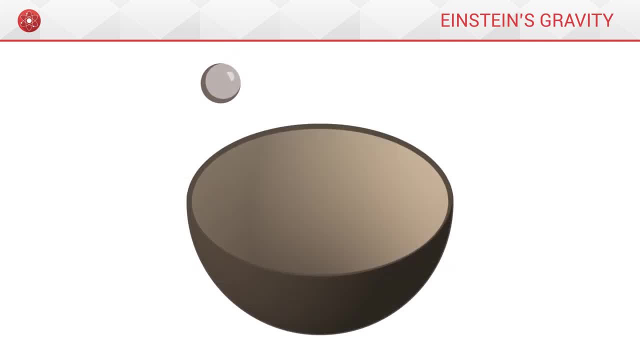 since it possesses a mass rather than A, since its mass is not as great. Let us now look at what happens if we release a marble in a bowl. Because of the bowl's curvature, the marble will slide along the inside of it until it. 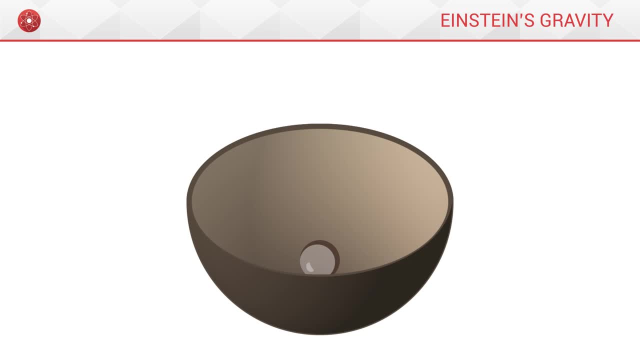 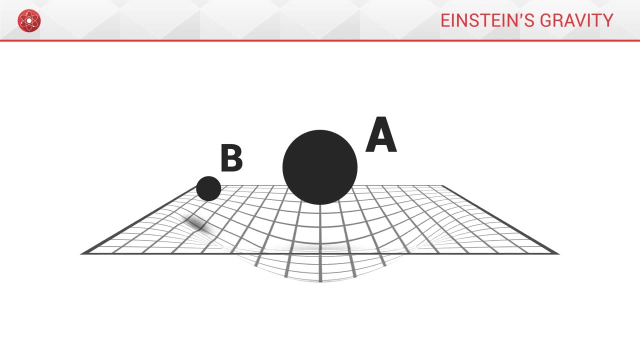 comes to rest at the centre. In a similar way, when we think about spacetime, in distorting the grid, A creates a sort of bowl around itself. Consequently, just like a marble, B will slide along this bowl gradually until it becomes. 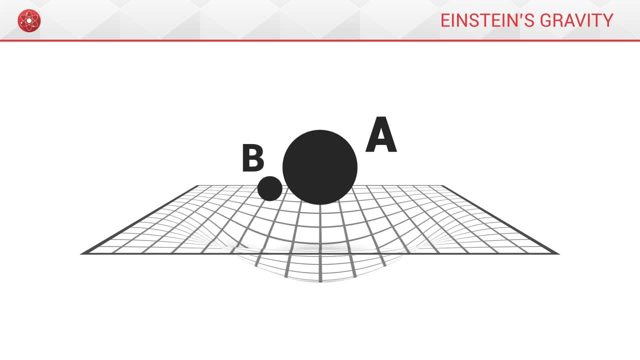 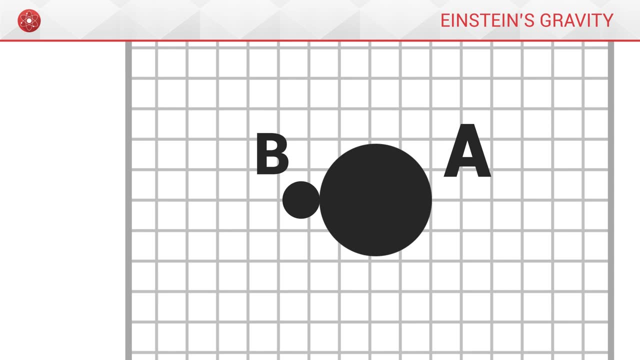 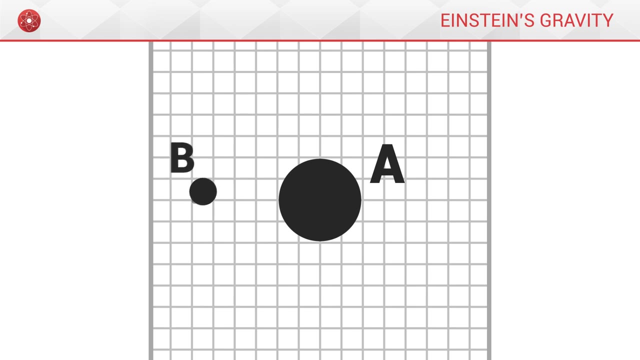 a mass. If we look at this scene from above, we observe that B is attracted by A, just like with Newton's model of gravity. Now, if we were to release B in this bowl with a certain speed, it would go around the bowl while getting closer to A.